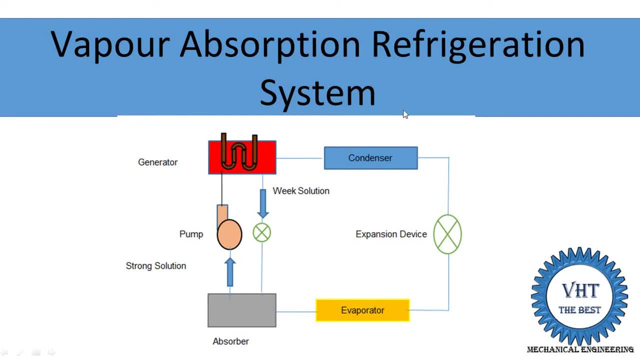 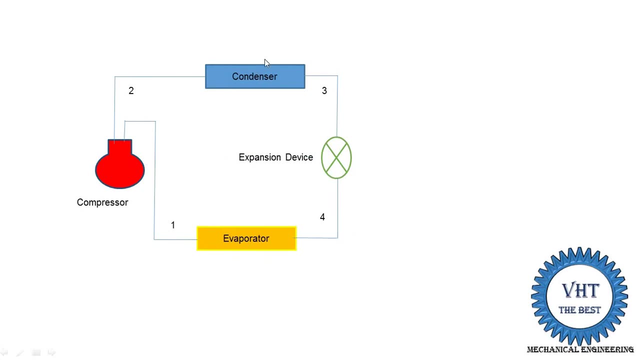 In this video I teach you the vapor absorption refrigeration systems. Introduction of vapor absorption, its working and various components I explain in this video. Now, before going to the vapor absorption systems, I just explain you the. what is the function of compressor in the VCRS system. 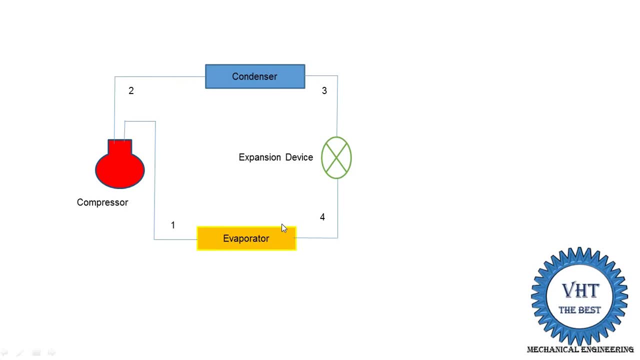 So this is the figure of the vapor compression refrigeration systems, In that you know the four components: compressor, condenser, expansion device and these evaporators. So, instance of the compressor, we use the three component into the vapor absorption refrigeration systems. 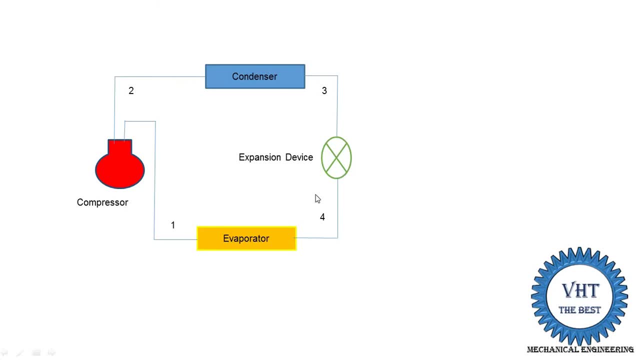 And another component is the same, that is, the condenser. expansion device and evaporator is already also present in the vapor absorption system, But instance of compressors, we use the another three component. we are not using the compressor in this systems. 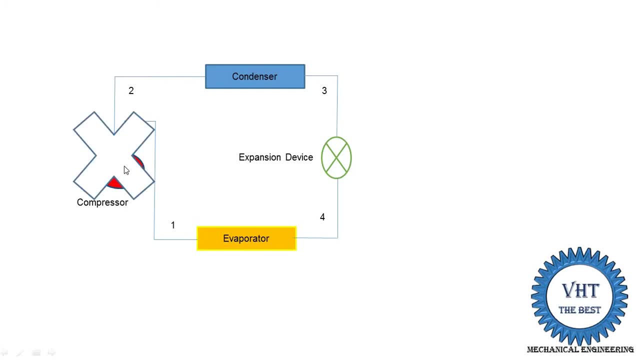 So by removing the compressor, we are need to put another device. So which device is putted and what is the reason of putting device? So the reason is that we have the three functions of the compressors in the VCRS system. 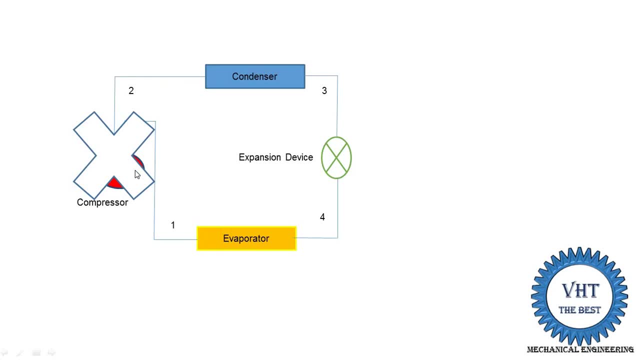 The first function is that it take the suction of the vapor refrigerant from the evaporator. So whatever the refrigerant coming from the evaporator, it suction into the compressor, Then in the compressor its pressure and temperature is increased. So it is the second function. 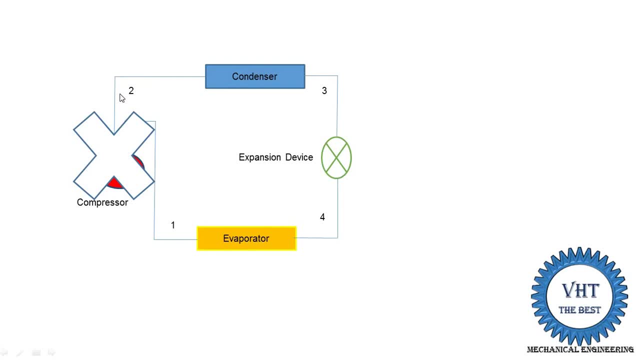 And third function is to deliver into the condenser. Now these three functions I am carrying out by three different functions In vapor absorption refrigeration system. So, instance of compressor, we use the absorber to absorb the refrigerants coming out from the evaporators. 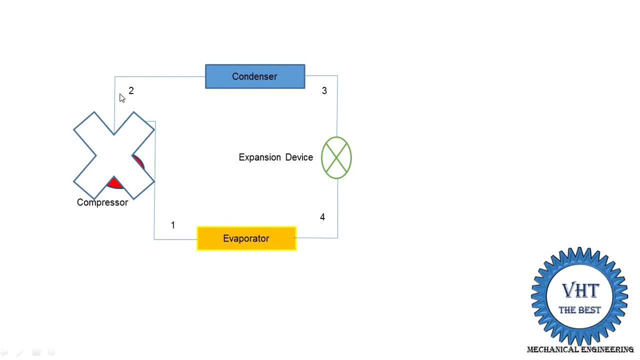 Increased pressure and temperature and supplied into the condensers. So let's move towards the VCRS system: vapor absorption refrigeration systems. So I put a already component that is present as compared to the VCRS system: the condenser expansion device and evaporator. 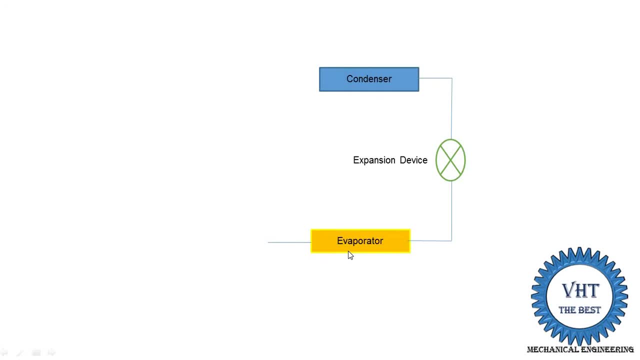 Now I tell you one another difference between VCRS and VERS, that in the VCRS system we use only the one substance, working substance or the liquid. That is only one and it is known as the refrigerants. Now, in vapor absorption cycles, we are using the two liquid. 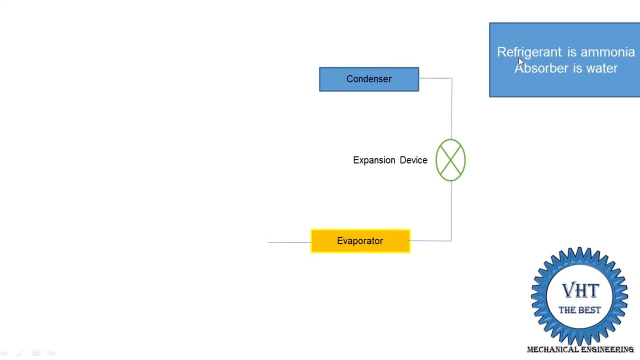 One is known as the refrigerants and second one is known as the absorber. Now, that is the number of pair- is used for a vapor absorption refrigeration system. This refrigerant and absorber is known as the parts, That is, the number of pair is available. 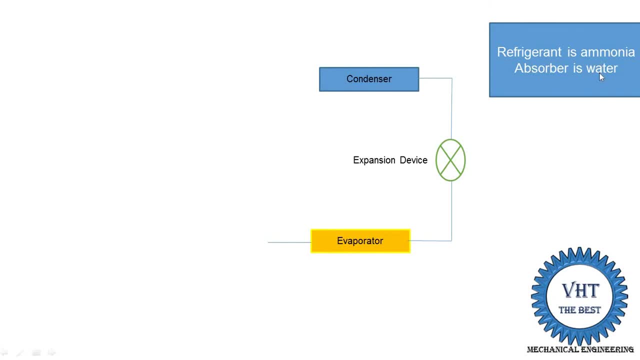 But commonly used pair is the ammonia and water. So deciding this pair- that is, the number of criteria- is there In this system. we use the ammonia as a refrigerant and absorber as a water. So this refrigerant is already circulated in condenser expansion device and evaporators. 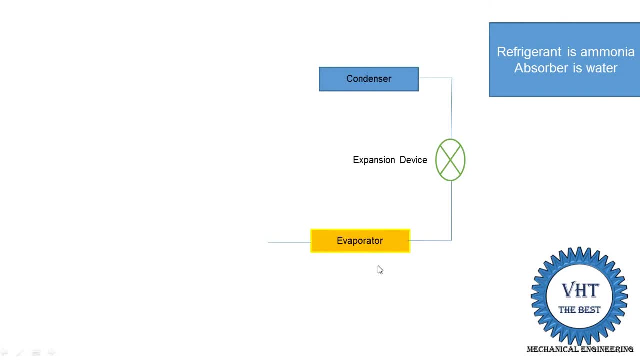 Same as the VCRS system Because to create the refrigerating effect in the evaporators we require the refrigerants. So refrigerant is circulated in condenser expansion device and evaporators. The absorber is not circulated in condenser expansion device and evaporators. 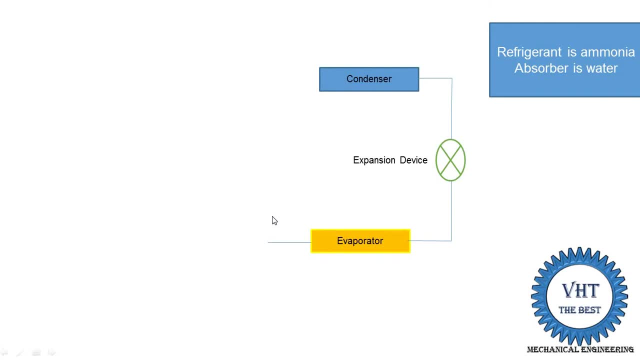 Now, the first function of the compressor is to take care the refrigerant coming out from the evaporators, And this function is carried out by using these absorbers. So in this absorber, water is available, Means, absorber, material water is used. 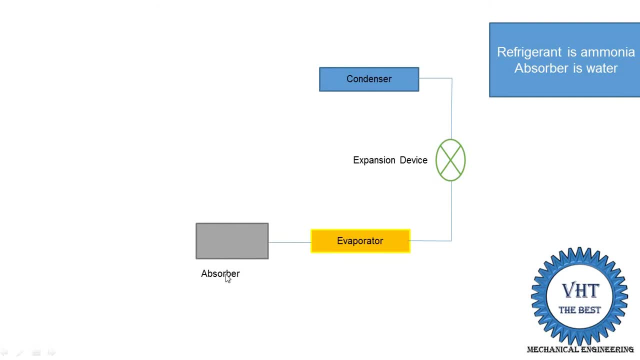 That is why water is available. If you are going in lithium bromide system, then as an absorber, lithium bromide is present. So it depends upon the system. But in system we use the ammonia and the water, Or it is also known as the aqua ammonia system. 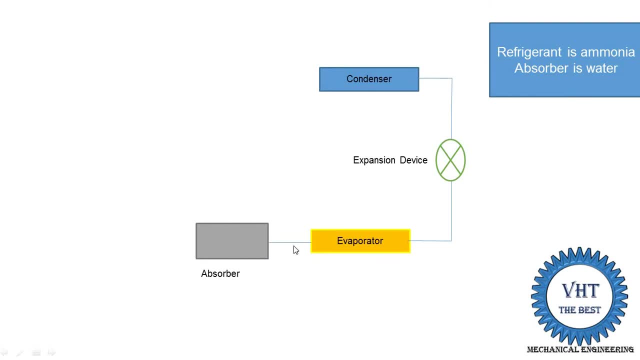 So if absorber, the water is already present. So whatever the refrigerant coming at the vapor state at the low pressure is coming to the absorber and it is mixed, And when it is mixed it creates the solutions. So when the absorber and refrigerant is mixed then it is known as the solution. 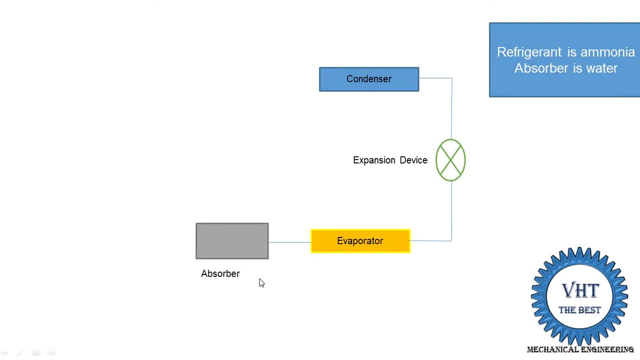 This absorption process is carried out by doing the cooling. So here the one heat exchanger is, provided that circulate the cooling water inside that and again it is coming out. And this is designed that the ammonia and water have a high solvability at the lower temperature and pressures. 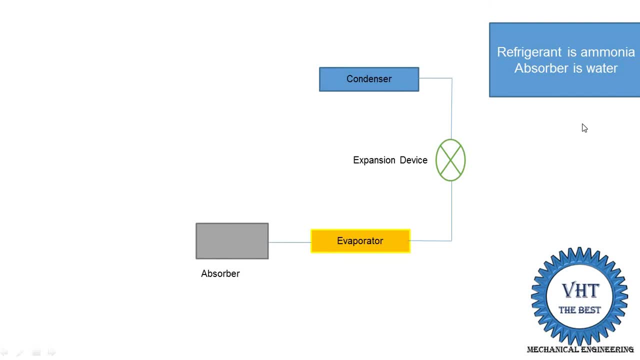 That means at the lower temperature they are easily mixed. That is known as the solvability. So they are mixed easily at the low temperature and low pressures And this create the strong solutions. Strong solution means it contains the higher percentage of ammonia or a refrigerant. 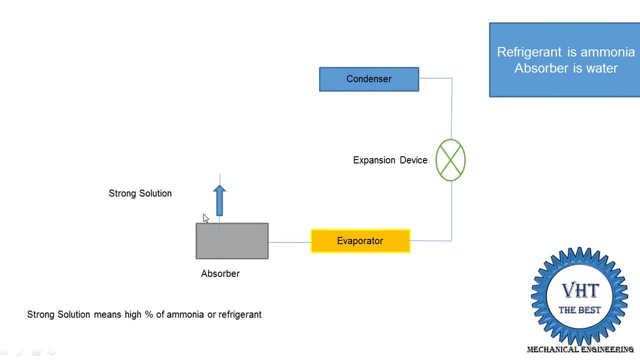 Means higher percentage of refrigerant is present than it is known as the strong solutions. This strong solutions is supplied into the generators by using the pump. So here we putting the one pump What the pump is doing. The second function of the compressor is to increase the pressure of the refrigerant. 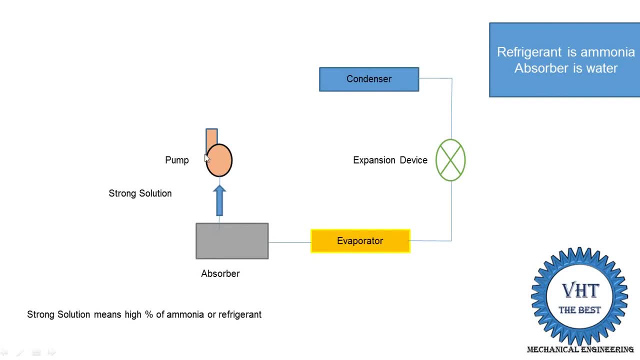 So pump is. similarly increase the pressures of the liquid refrigerants. So pump is used to increase the pressure of the systems Up to the pump is increased the pressure up to the 10 bar, Then it is supplied into the generator That this strong solution is supplied into this generators. 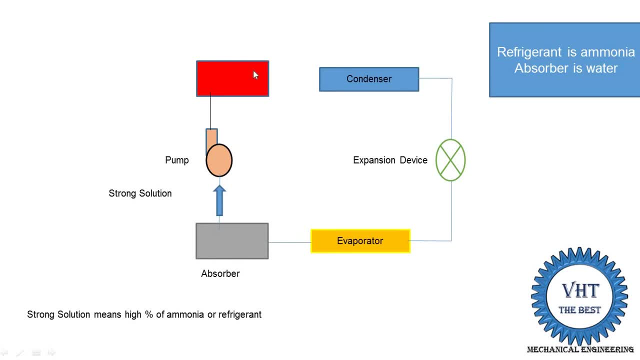 This generator is not convert the mechanical energy into electrical energy. This is not type of that generators. This generator is the device in which we are supplying. We are supplying the heat energy. So for supplying the heat energy, we are putting here the generators. 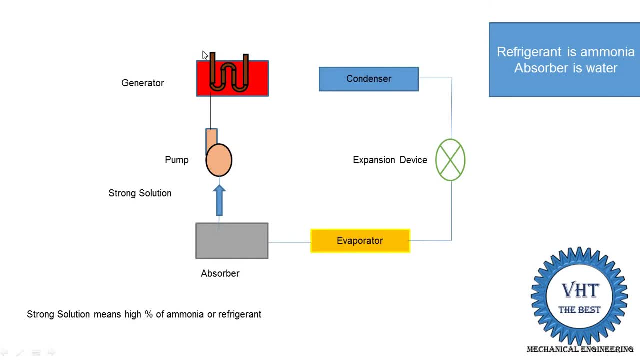 These generators may be electric heater, may be steam or may be gas or a waste gases coming out from the industries. So it may be electric heater or the waste steam coming out from the industry That is also supplied inside the pipe and that also gas. 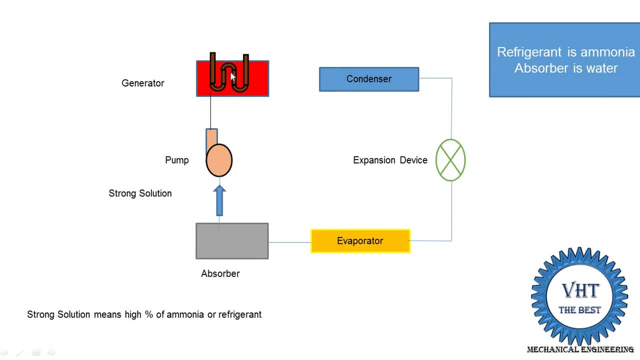 It is also be available solar energy. So simple thing is that in generator, We supply the heat energy to this strong solution. This strong solution is mixture of aqua, ammonia means ammonia and the water. Now, when we supplying the heat to this strong solution or these mixtures, 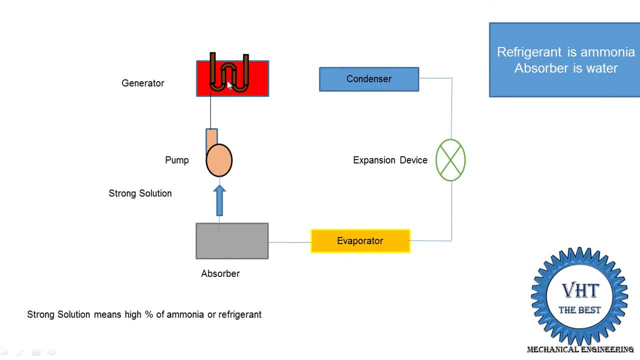 They are try to separates So they are selecting on the basis of that. they have a different boiling temperatures, So refrigerant have lower boiling temperatures and absorber as a higher boiling temperatures, So lower boiling temperature, refrigerant is used. That why it is start to boil earlier than the absorbers. 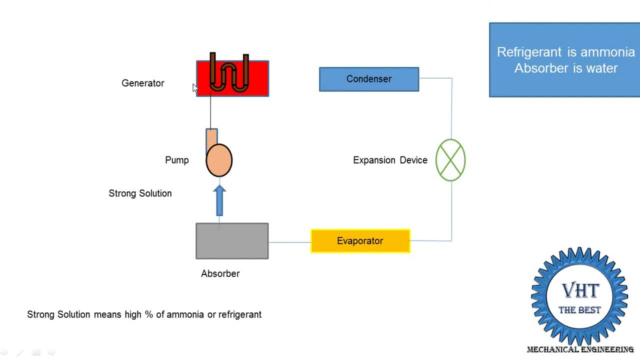 And it is designed such a way that it is have high separativity at the higher temperature and pressure. So they are separated easily at the high temperature or lower solvability. It is called lower solvability at the higher pressure and temperatures. 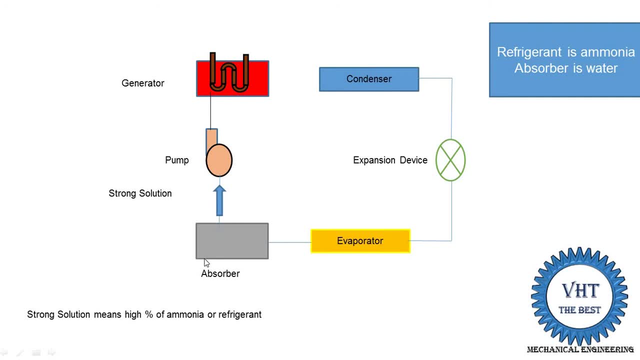 And higher solvability at the low temperature and low pressure in the absorbers. So at that high temperature It is separated and what amount of the ammonia coming? That is up to the 88% ammonia is separated in the generators, Then it is supplied into the condensers.